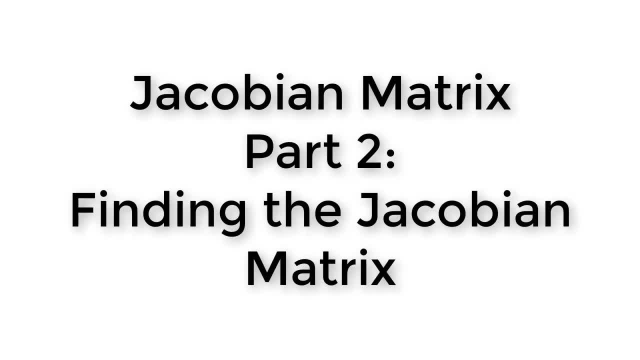 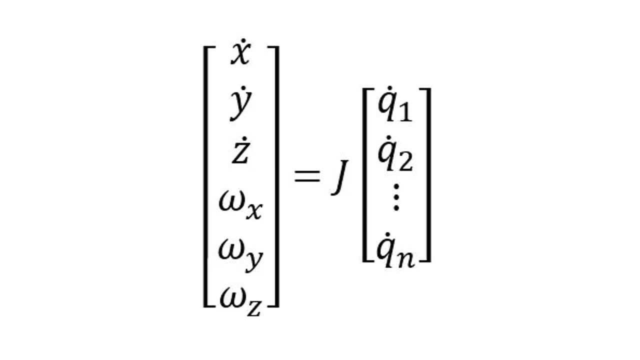 In the last video we learned that the Jacobian matrix defines the relationship between joint velocities and end-effector velocities in this way. Now we know that each q is a joint variable, so that means that the J matrix needs to have a number of columns equal to the number of joints in the manipulator. 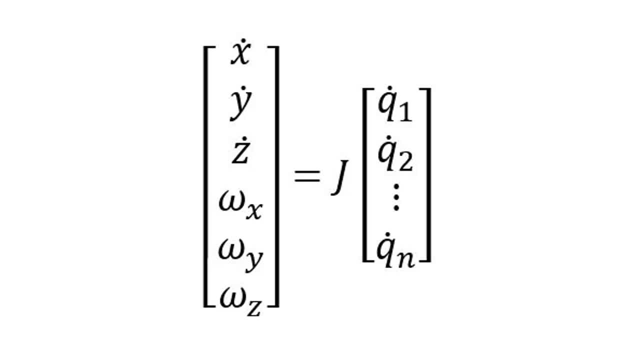 And since there are six things in the vector on the left, that means that the J matrix needs to have exactly six rows always. So, for example, suppose that we are trying to find the Jacobian matrix for a manipulator with three joints, two revolute and one prismatic, like our Scara manipulator. 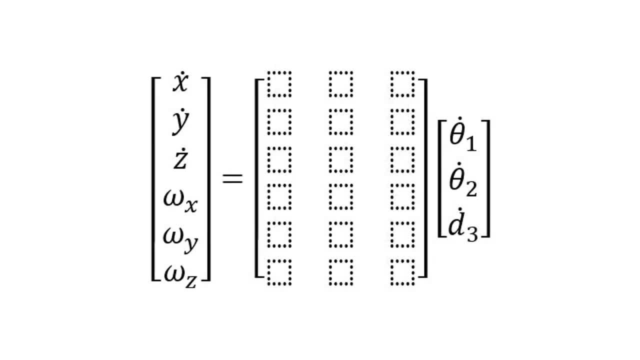 The equation would look like this. Now we need to find what goes on in the Jacobian matrix. We need to find what goes in each of those six rows and three columns of the Jacobian matrix. Now the way we do this is by using a table that tells us how to fill in each column. 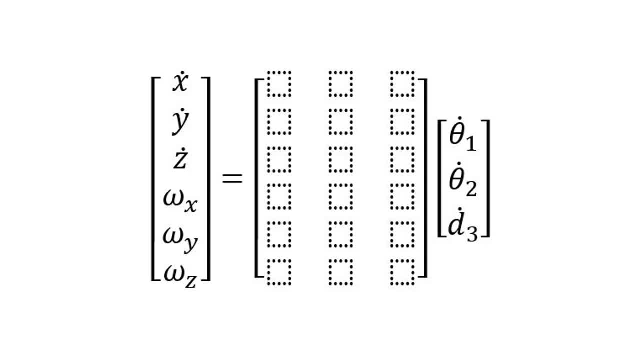 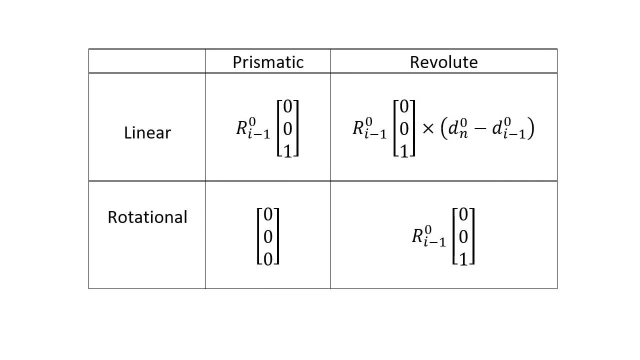 First I'm going to show you what the table looks like and then we'll see how to use the table. The table looks like this. Notice that there are two rows in the table. The top row is for determining the linear parts of the end-effector velocity. 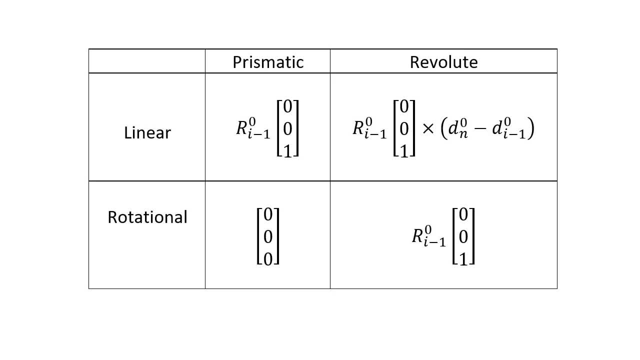 And the second row is for finding the rotational parts of the velocity. There are also two columns. The first column we'll use any time there's a prismatic joint, And the second column we'll use any time there's a revolute joint. 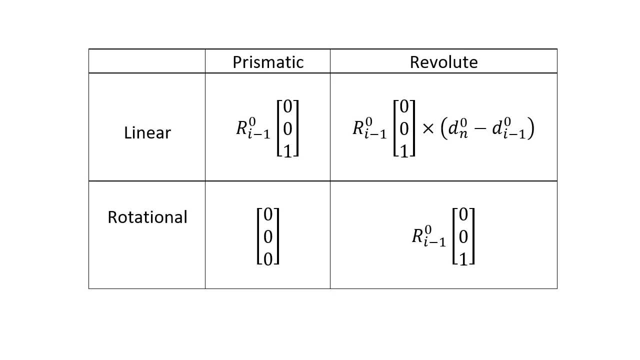 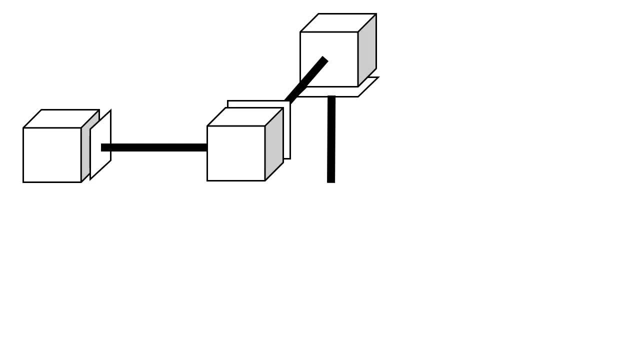 Let's learn how to use this table by using an example. For the first example, let's suppose that the manipulator has all prismatic joints like this. Now we know that our Jacobian matrix will look like this, with 3 d's in place of the q's on the matrix. 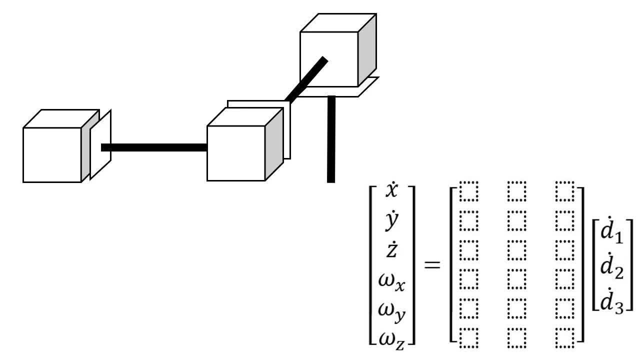 because we only have 3 prismatic joints. To find what goes on in each of the Jacobian matrix places, we'll use the table. We'll start with the first column. The first column of the Jacobian matrix is for the first joint of our manipulator. 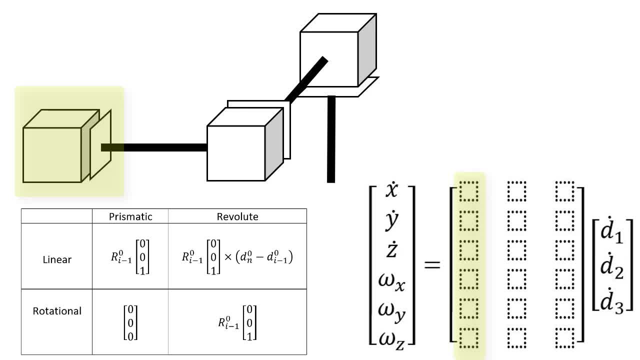 and that first joint acts on a prismatic one. So we get this as things in the prismatic part of the table. The I in the table refers to which joint we are looking at. This is joint 1, so I is equal to 1. here We can fill in the first column. 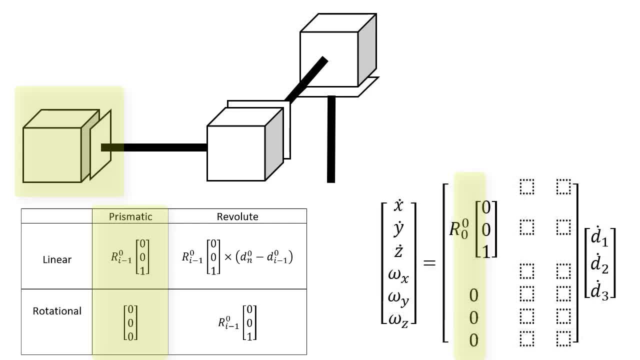 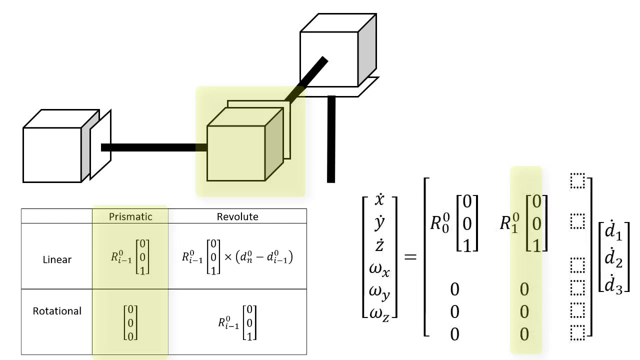 of the table like this: Now, the second column of the Jacobian matrix is for the second joint, joint 2.. So I equals 2.. We get this stuff from the prismatic part of the table again, because this joint is also prismatic, And we fill it in like this: Finally, we do the 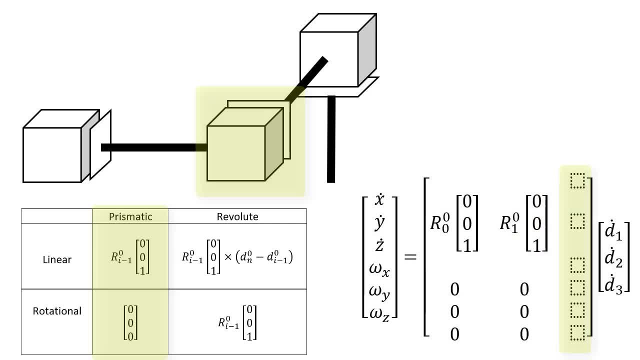 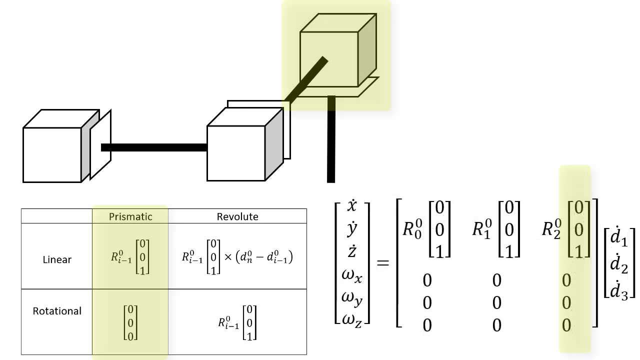 third column of the Jacobian matrix. The third joint is also prismatic, so we get this stuff from the prismatic part of the table again. Here I equals 3, because this is the third joint. So we fill in the third column like this. Now we're not quite done yet, because we've 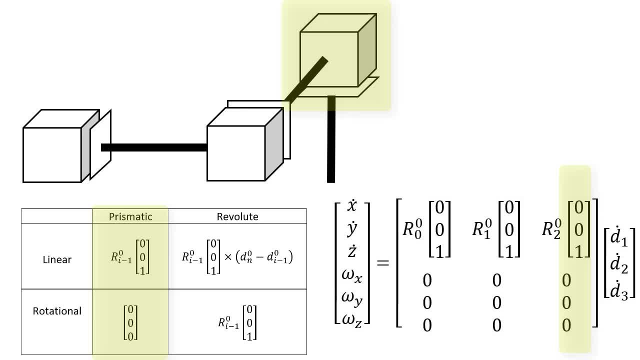 left some variables in this table that we can fill in. I bet you recognize the R matrix notation. We learned all about this in Robotics 1.. R00 means the rotation from frame 0 to frame 0.. R01 means the rotation from frame 0 to frame 1.. 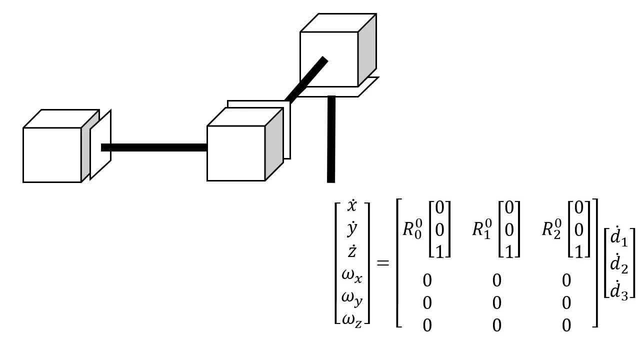 And R02 means the rotation from frame 0 to frame 2.. To finish this Jacobian matrix, we need to find these rotation matrices and fill them in. So let's look back at our kinematic diagram and put frames on it. We already learned how to do this, so I won't go through that. 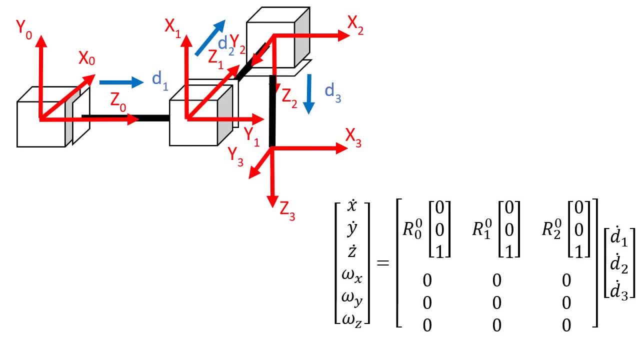 again here. Okay, so R00 means the rotation from frame 0 to frame 0. That means that we can't do any rotation from frame 0 to frame 1.. So R00 will always be the identity matrix, which means no rotation. In our Jacobian matrix we need to multiply this matrix times the. 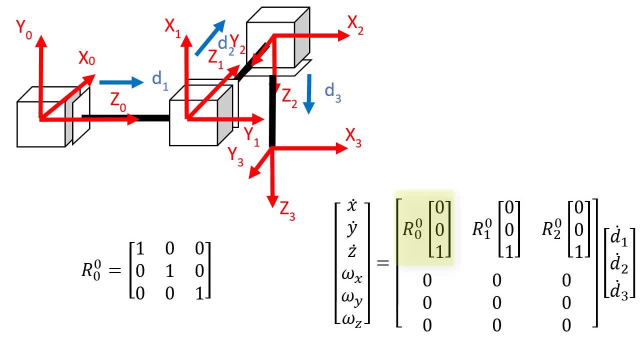 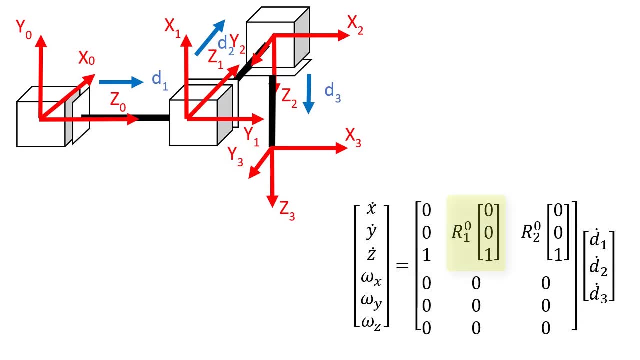 vector 001, which is actually the exact same thing as just taking the third column. So I'm going to take the third column of R00 and fill it into the Jacobian matrix. Now we're going to multiply this matrix by the vector 001.. We've also done this a bunch of. 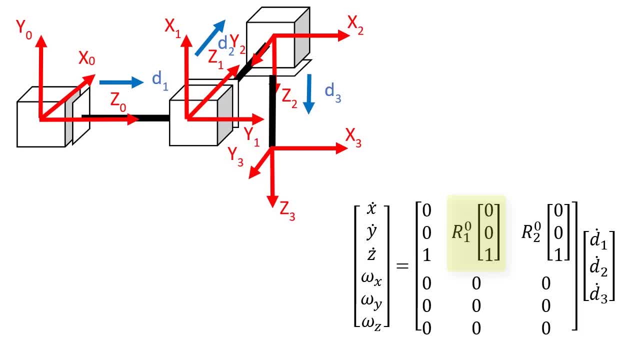 times in the past so I won't go through how to get this again. R01 is this? Now, since multiplying this matrix by the vector 001 is the same as just pulling out the third column, I'm just going to take the third column and plug it into the Jacobian matrix, like. 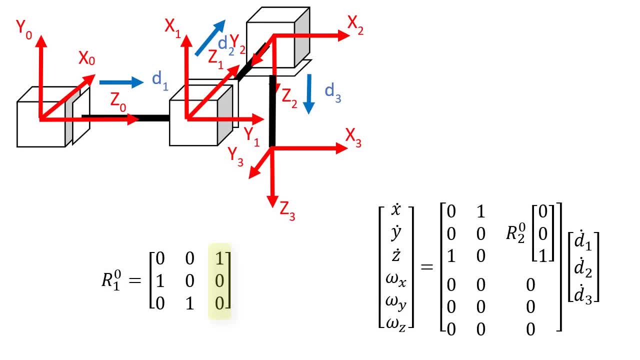 this. Lastly, I need to find R02.. Think back to Robotics 1 and you'll remember that we can do this by multiplying: R02 equals R01 times R12.. I've already found R01, so now I just need R12.. R12 is this Now? 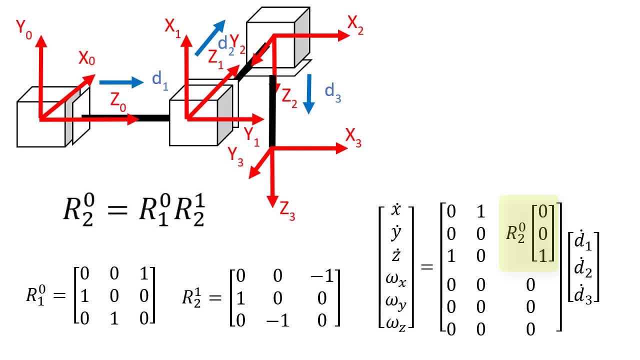 I multiply R01 times R12.. Now my defaultToSt括Line is it's size, andviewerSteverTheantly pasó this jakby to get r02 as this. I pull out the third column because I need to multiply this by the vector. 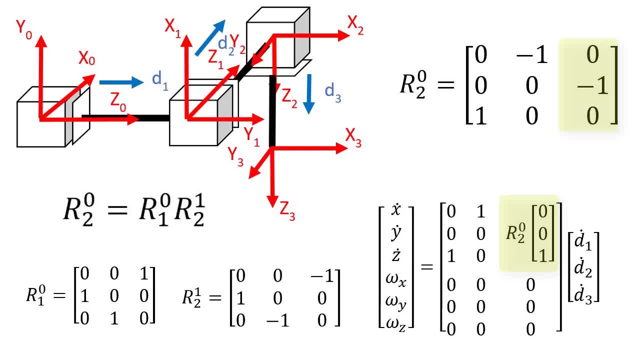 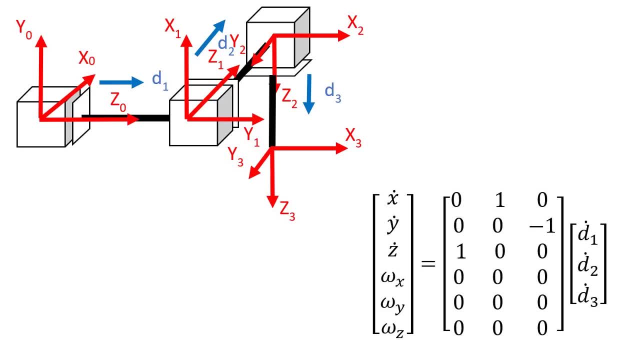 001, and then I stick it into the Jacobian matrix. And this is the final Jacobian matrix. Before we move on to another example, let's think about what this matrix means and what we've learned about the velocities. Now I can multiply through to get 6 equations. 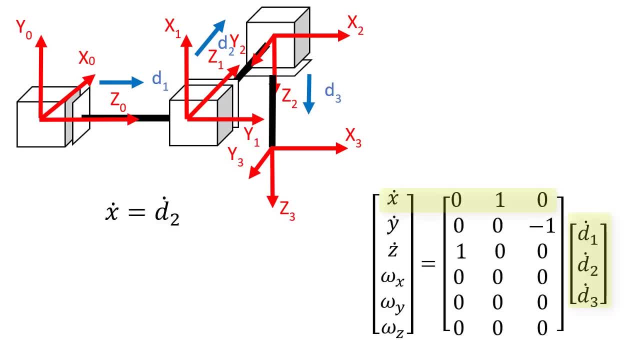 My 6 equations say: x dot equals to d2 dot. Y dot equals to negative d3 dot. Z dot equals to d1 dot. Omega x equals 0.. Omega y equals 0.. 徐 equals 0.. WER equals 0.. 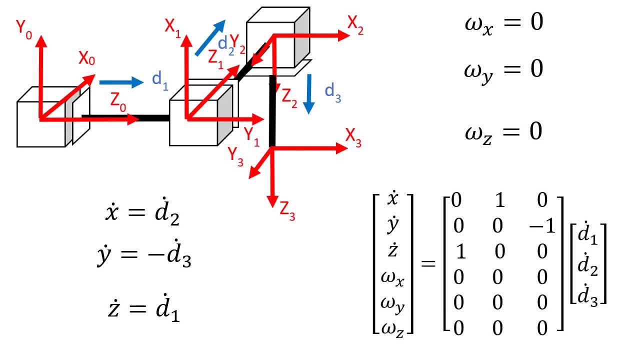 0 and omega z equals 0.. Does this make sense? Let's look back at our kinematic diagram. The first equation we have here says that x dot is equal to d2 dot. According to our equations, the speed of the end effector in the x direction is equal to the speed of the. 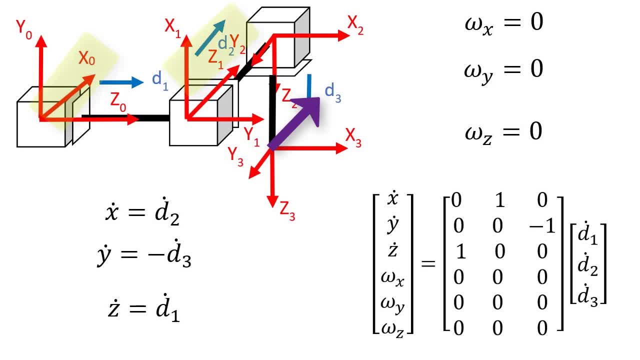 second joint. Does that make sense? It does, because the second joint is pointing entirely in the x direction and it always is, no matter what happens with the different joints. It's true that the velocity of the end effector in the x zero direction is completely controlled. 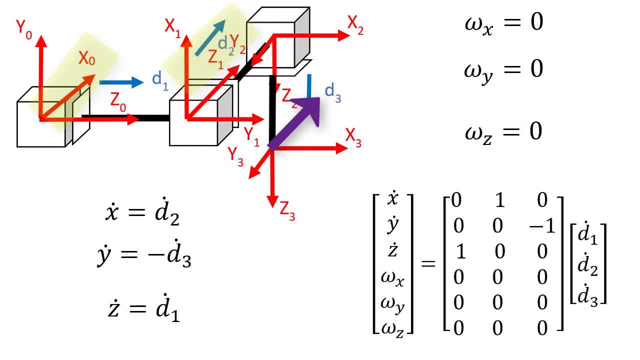 entirely, only by the second joint. Our second equation says that y dot is equal to negative d z. This equation is a positive 3 dot. Does that make sense? The y direction is up and the d 3 direction is pointing down. 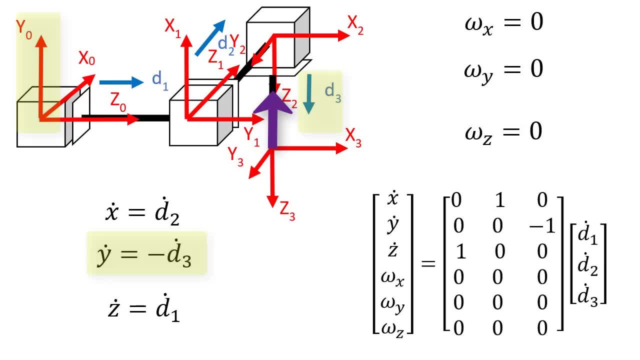 Our equation is telling us that the velocity of the end effector in the y direction is equal to the opposite of the speed of the third joint. and that's true here. The velocity of the end effector in the y direction is completely controlled only by joint 3 and 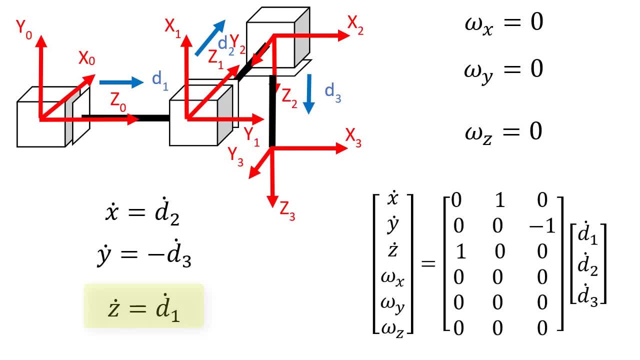 no other joints. Our third equation says that z dot is equal to d1 dot. Does that make sense? It does, because z is pointing in this direction and the first joint is moving in that same direction. So the speed of the end effector in the z direction is completely controlled. 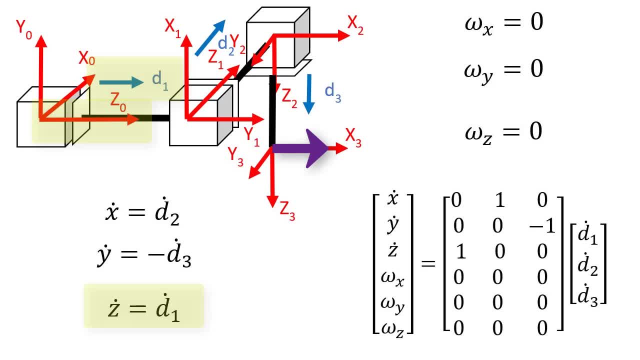 only by the first joint. and when the first joint is moving in the positive direction, the velocity of the end effector in the z direction is also positive. What about these other three equations that say that omega x is 0,, omega y is 0, and omega? 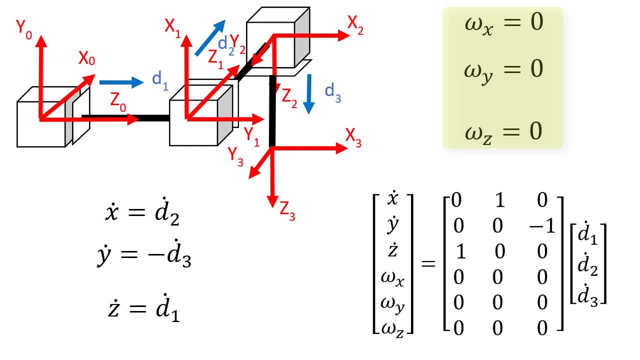 z is 0?. These equations are telling us that, no matter what we do with our three joints, we can't get the end effector to rotate around x, y or z. Is that true? It is because in our manipulator we only have prismatic joints. There is no. 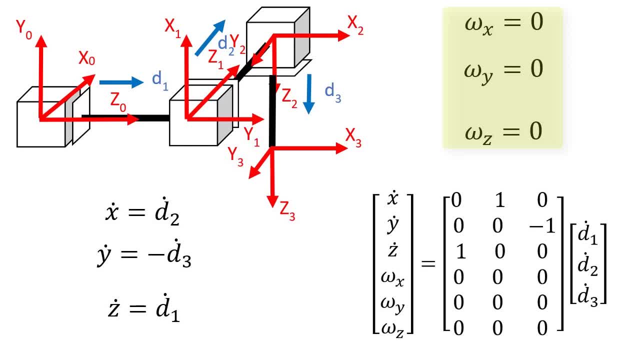 way for us to get our end effector to rotate. For example, imagine we had a gripper attached to this end effector. Could we get the gripper to point in a different direction? No matter what we do with these three joints, the gripper will always be pointed in the same direction. 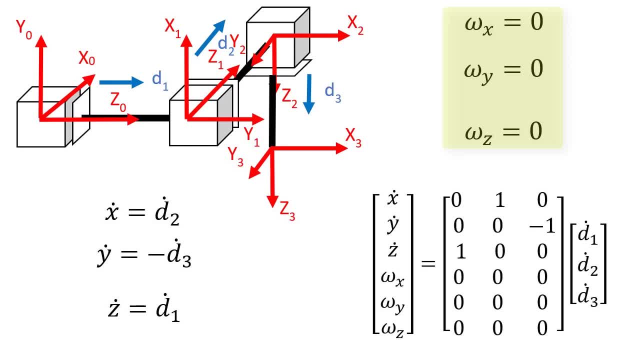 – there is no way to rotate the gripper. So These three equations seem to match our kinematic diagram. also, Let's do another example. This time let's do an example with two revolute joints like this. Here our Jacobian matrix will still have six rows, because the Jacobian matrix always has. 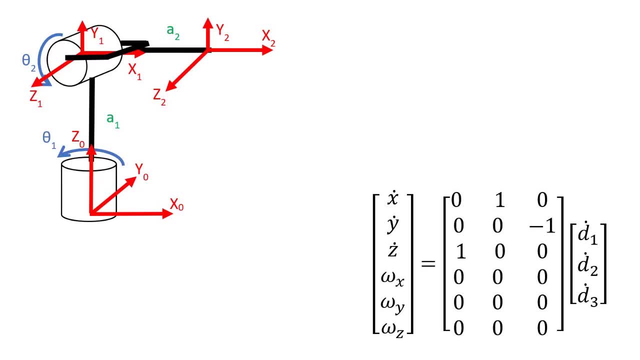 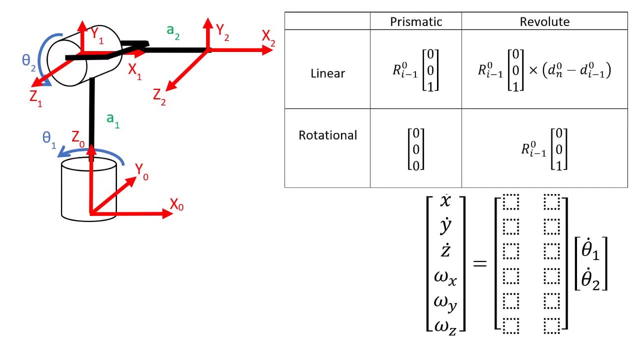 six rows but it will only have two columns because we only have two joints here To find the Jacobian, we'll start by going to the table and getting the part that is for a revolute joint, because our first joint is revolute. 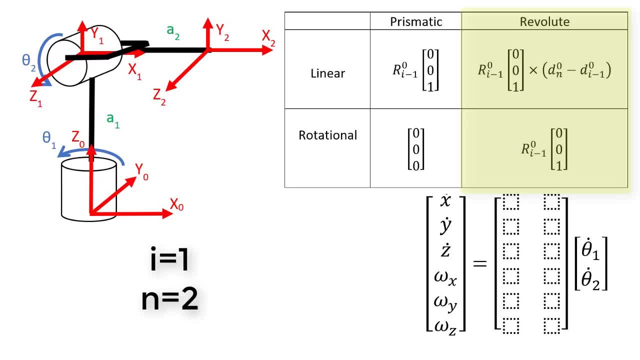 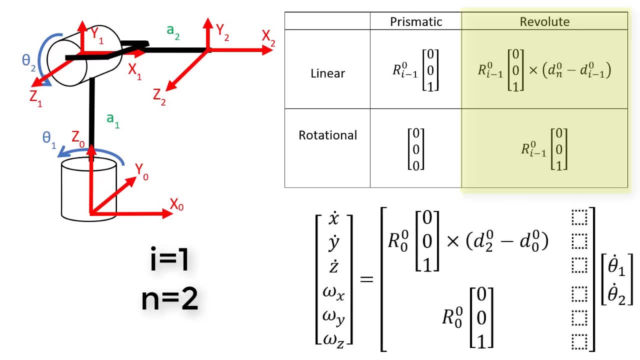 Now i here is 1, because this is the first joint that we are working on, but n is going to be 2, because there are a total of two joints. So we fill in the first column as R, 00 times the vector crossed with the displacement. 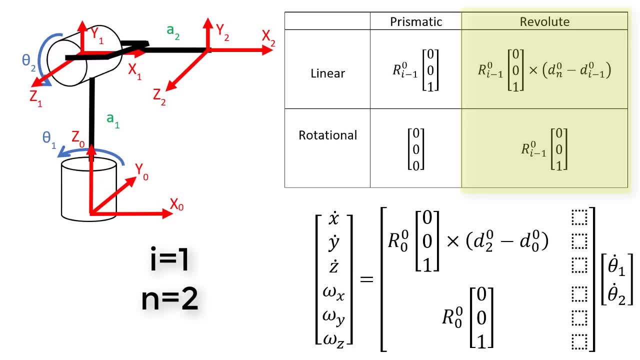 from the center of frame 0 to the center of frame 2.. Minus displacement from the center of frame 0 to the center of frame 0, and then down here we put times, the vector. That will be the first column of our 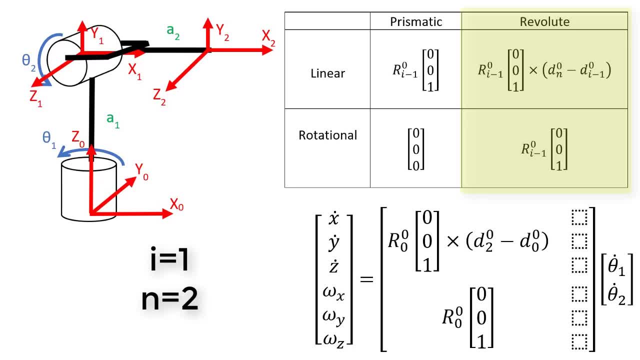 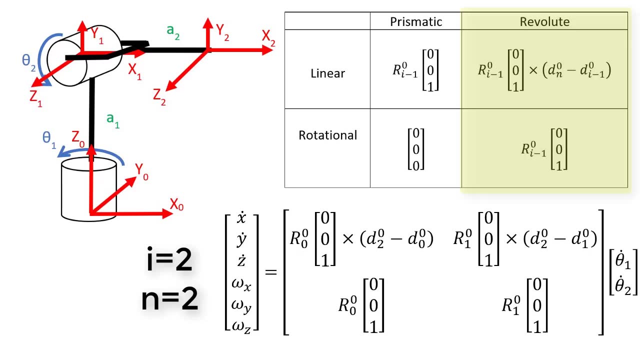 Jacobian matrix. For the second column we'll have to use the revolute part of the table again, because our second joint is also revolute. So we'll fill in the second column like this: R01. since this is the second joint, I is now equal. 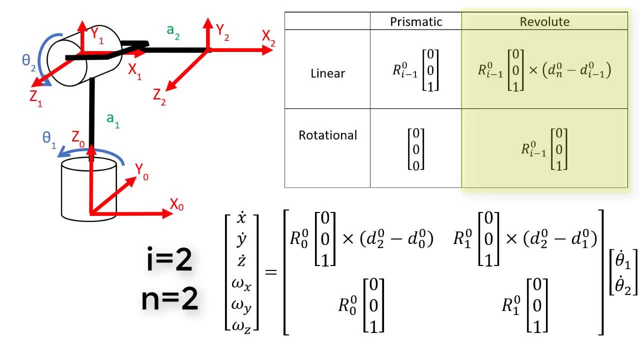 to 2, times the vector crossed with d02 minus d01.. In the bottom part of this column we'll put R01 times. Now let's go back and start to fill in the parts of this table. R01 equal to 0: 1. 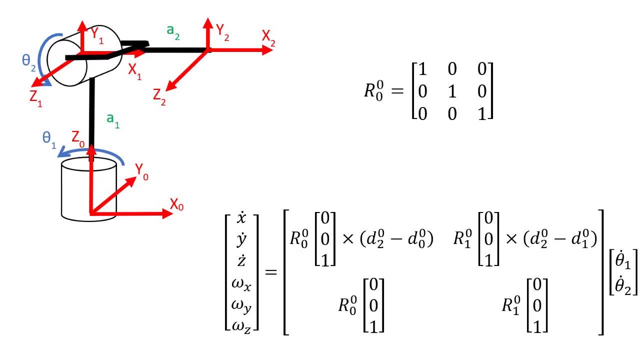 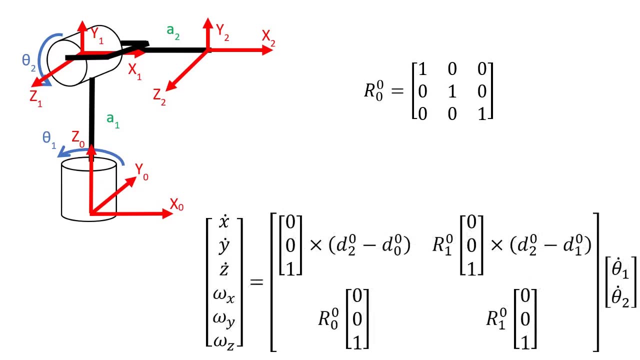 R01 equal to 1, 2, R is easy, it's just the identity matrix, since there's never any rotation from frame 0 to itself. So we take the third column of this matrix and this whole expression becomes the vector. Now, what about d? 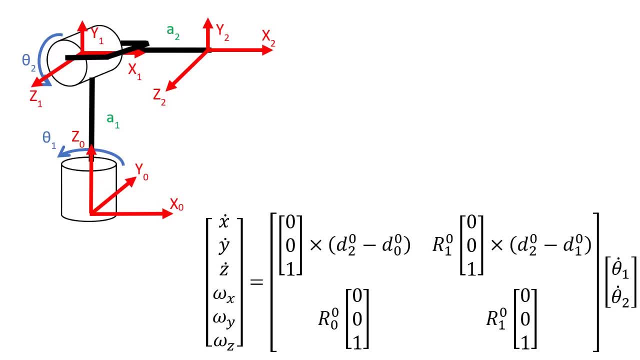 How could we get that? Well, we know that if we have the homogeneous transformation matrix, the upper left-hand part is the rotation matrix and the upper right-hand part is the displacement vector. We can find d by first finding h and then taking the upper right-hand part of 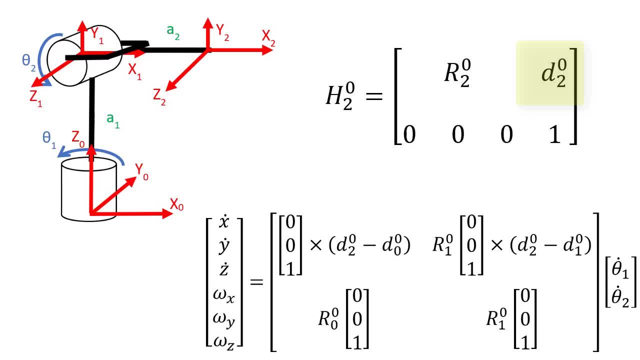 that matrix. Since you already know how to find homogeneous transformation matrices, I'm not going to go over that again here. If you use the Denevet-Hartenberg method or any other method to find the homogeneous transformation matrix from frame 0 to, 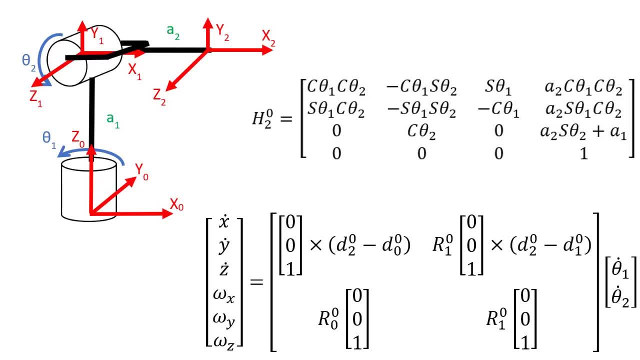 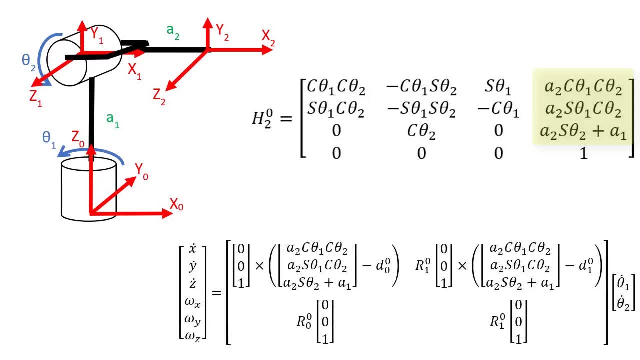 frame 2, you'll find that it is this. D is now the upper right-hand corner, so I'll extract that part of the matrix to fill in here. D is easy because the displacement from the center of a frame to itself is always. 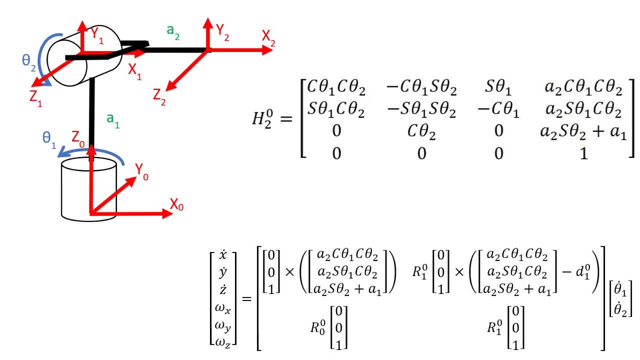 zero. Now I have to take the cross product of these two vectors. If you don't remember how to take a cross product, then you're watching this video on my website, RoboGrakcom. There will be a link next to this video to help you remember how to take the cross product. 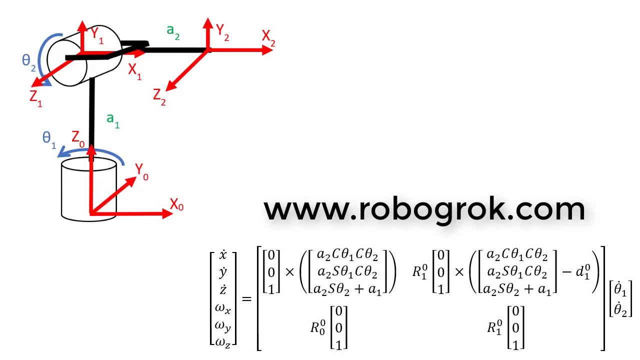 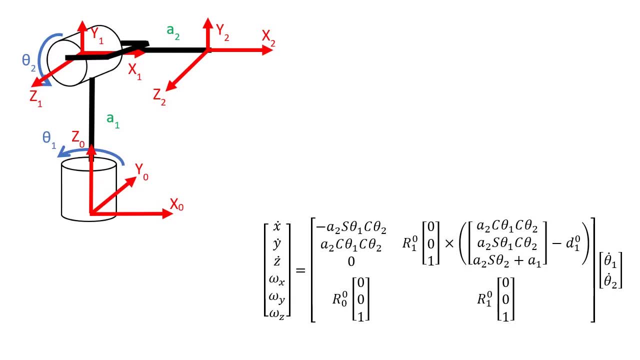 of two vectors. After you take the cross product, the result that you get is this: And we're done with this part of the table. Now for the second part of the table. we have r zero zero times zero zero. one r zero zero is this: 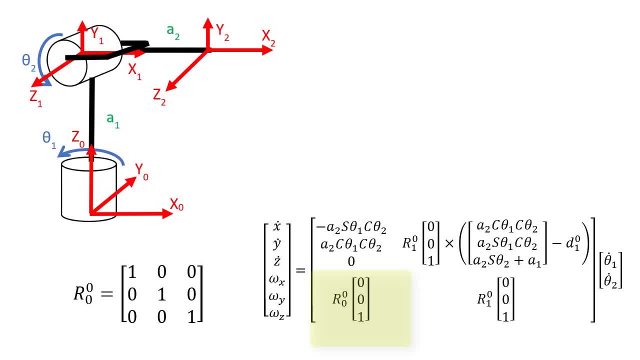 The identity matrix, and so we take the third column of that and fill it in here. Next, let's do the second column of the Jacobian r, zero one is this: I take the third column and fill it in. And d zero one is this: 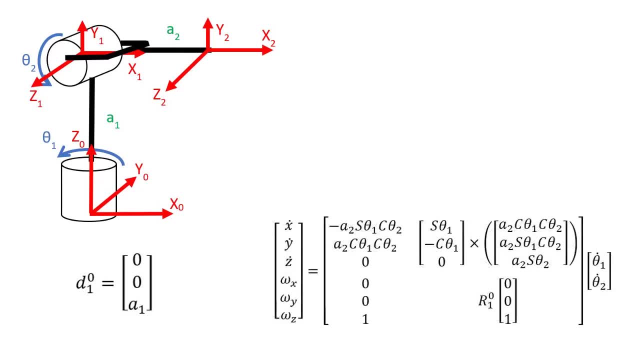 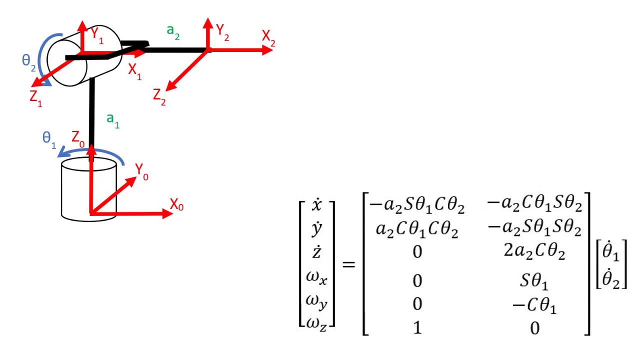 I do the subtraction and then I take the cross product of these two vectors and fill it in to my Jacobian matrix. For the bottom part, I take r zero one and I take the third column and fill it in. So I'm done with the Jacobian matrix. 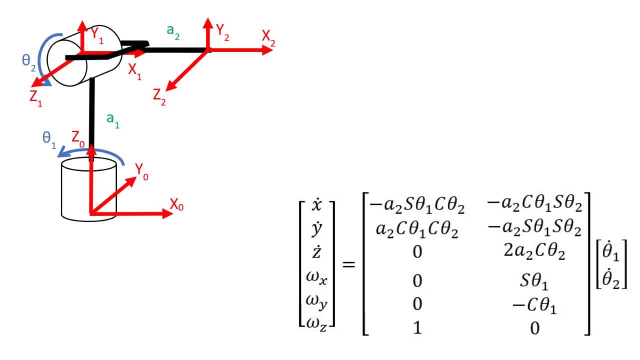 Before we finish this video, let's take some time to think about what this Jacobian matrix means and check to see if we're correct. Multiplying this out gives us six equations, as shown here. First, Note that All of these velocities are zero all the time. 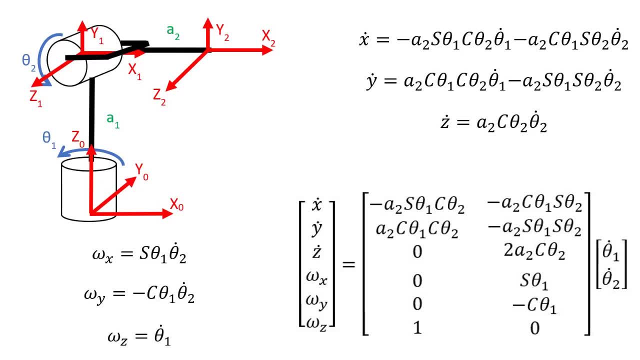 We could make any one of these velocities become non-zero by moving either theta one or theta two, But some of the velocities do depend entirely on only one of the two joints. For example, the speed at which the end effector rotates around the z zero axis is equal to. 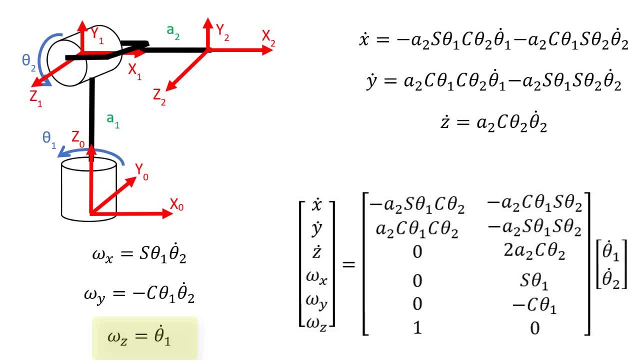 theta one dot. The speed at which the end effector rotates around z zero is equal to theta one dot. It doesn't depend at all on the speed of theta two. Examining our kinematic diagram, we see that this is true. We can make the end effector rotate around z by moving theta one, but we cannot make 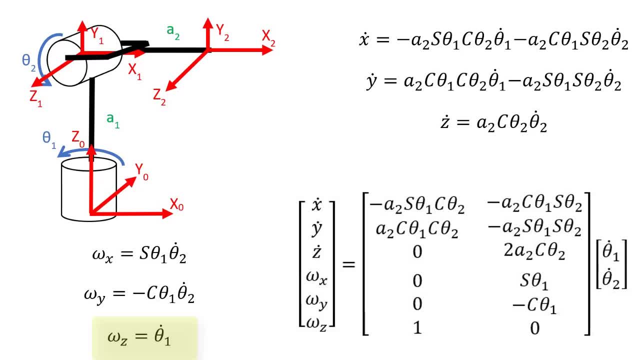 the end effector rotate around z zero by rotating theta two. Theta two only makes the end effector rotate around the x Or the one y-axis. In fact, by looking at our Jacobian matrix, we see that the speed of rotation 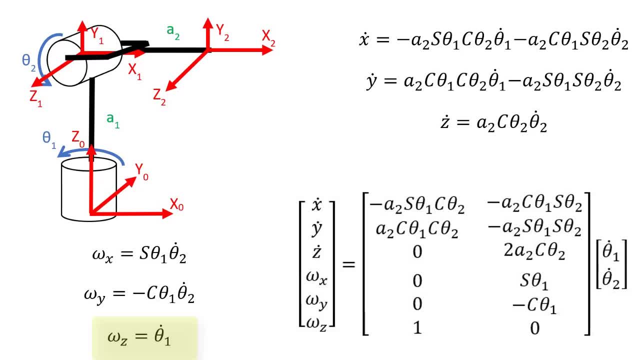 of the end effector around the x- and y-axis depend only on the speed of joint 2, not the speed of joint 1.. They depend on theta 2 dot but they do not depend upon theta 1 dot Also. 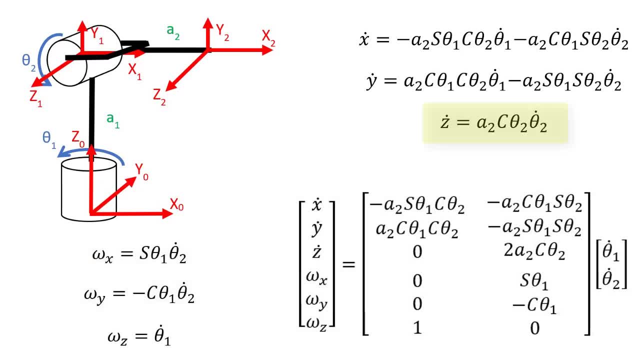 the linear velocity of the end effector in the z-direction depends only on theta 2 dot, not on theta 1 dot, And looking at our kinematic diagram we can see that this is true. Moving theta 1 does not make the end effector rotate around the x-axis or the y-axis, nor does